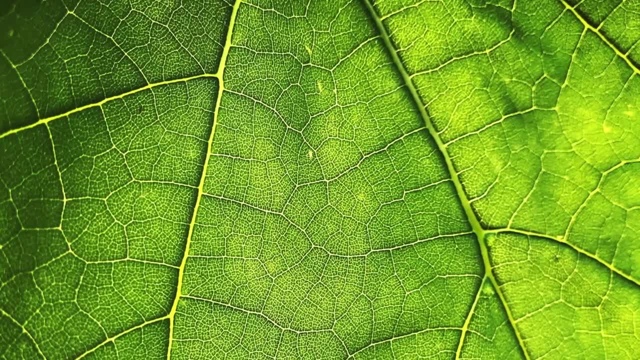 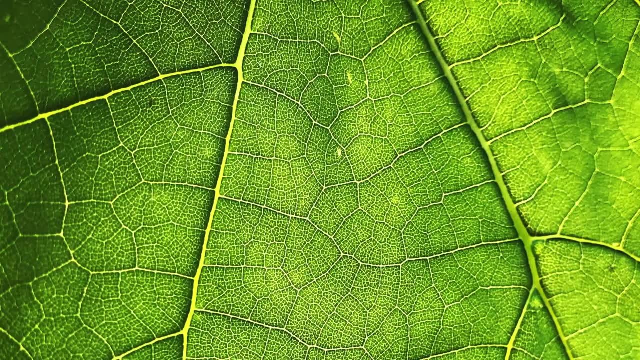 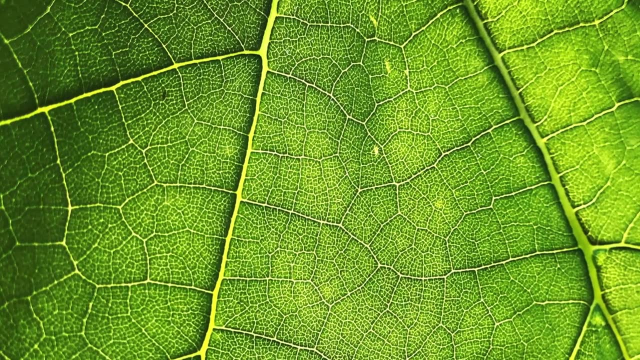 I mean, we probably know, you know from all the commercials in childhood, that calcium is required for our bone makeup, but it's also required for cell integrity, the strength of the cell wall, And because of that, because of that, that structural 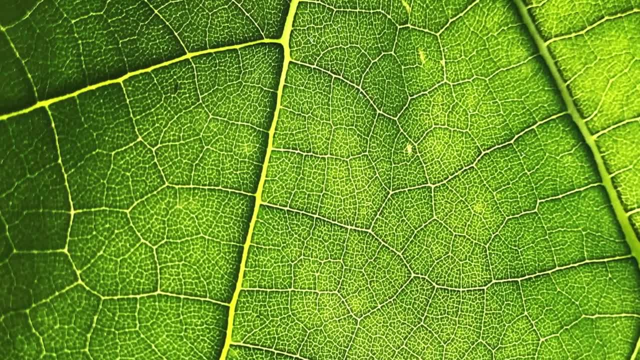 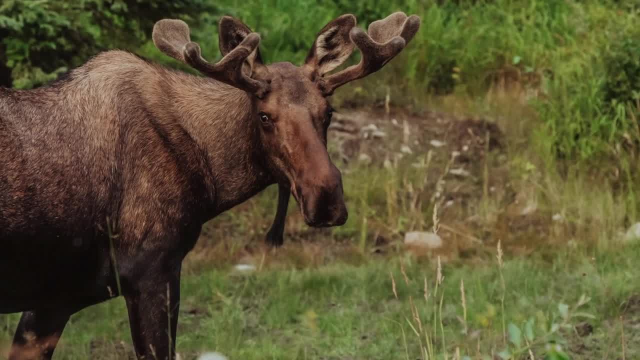 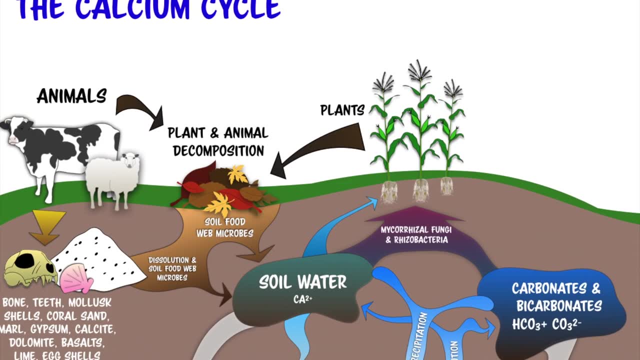 quality of calcium. it's needed in the right forms for plants and animals all life to be healthy, And so we need to make sure that our calcium is cycling, that we understand calcium well, because calcium is so important, And without adequate levels we will not have proper. 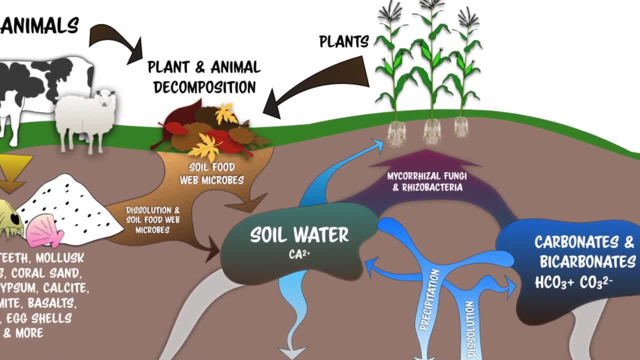 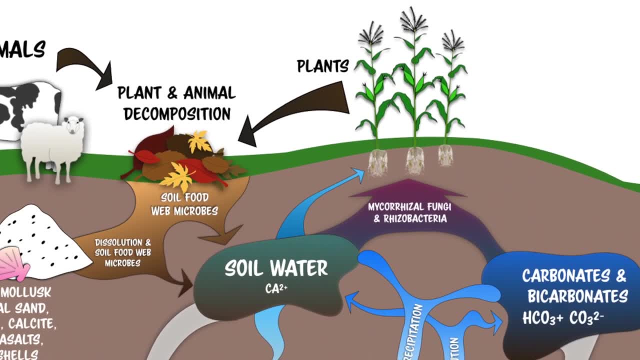 plant performance. So when people talk about, you know, fungal blights and all these things infecting their plants, a lot of the time it's because the cell wall's integrity is breaking down. The calcium pectin in the cell wall is breaking down, And so we need to make sure that. 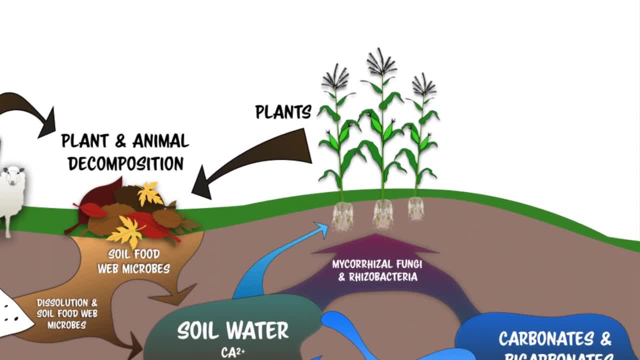 they're doing the right thing to the plants we treat for plants and animals. So, yeah, in this new world that we're going through right now, we're seeing the growth ofasons And so one of the pieces that thisенный industry experiences. 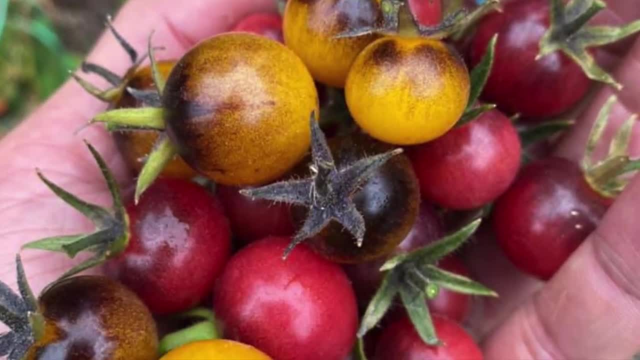 if you compare that to the other sensors that we have, is the growth. of the Juvel is really here. Here we've— for instance, you can look at República consumers. we have a fighter company which is known—although it's actually a Magazin. 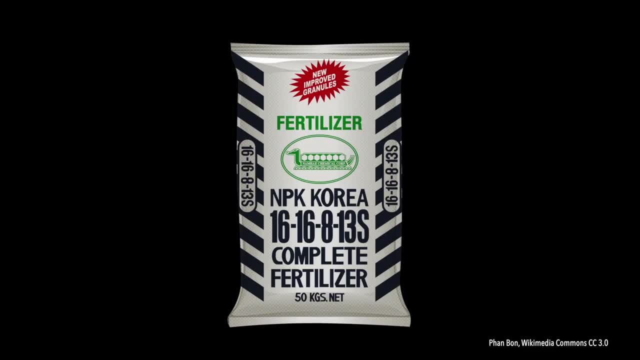 it's still a company, it's not fully established—they're there, but they're there and they're saying: we didn't like workouts, They're no longer in training. You can move up, you can do whatever you want. everything works like�. 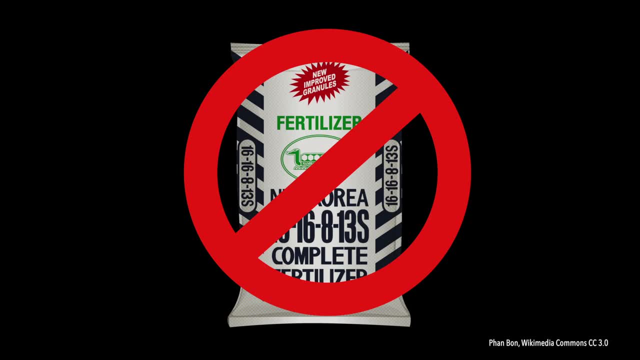 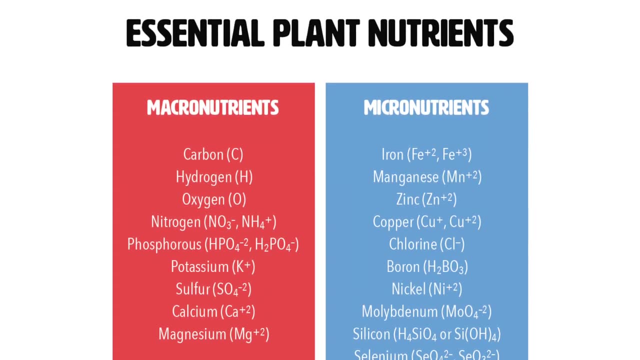 But yeah, there are available solutions, but they don't work for companies around the world tremendely self-evidentast haciendo son depositos. maybe arguably more important though, all of these things are required, there's no hierarchy of need, really. there's hierarchy of access, sometimes for certain, certain processes. right, we need this. 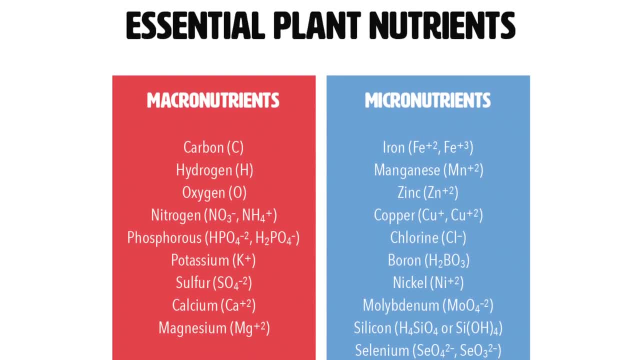 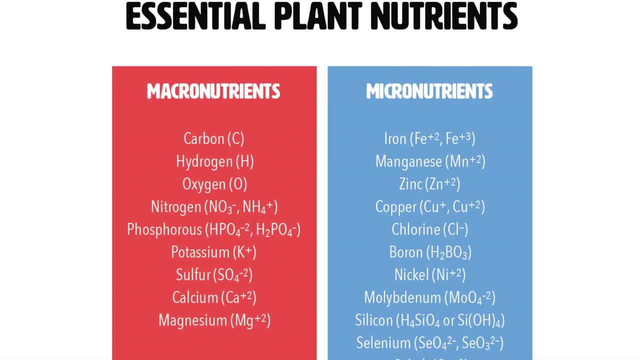 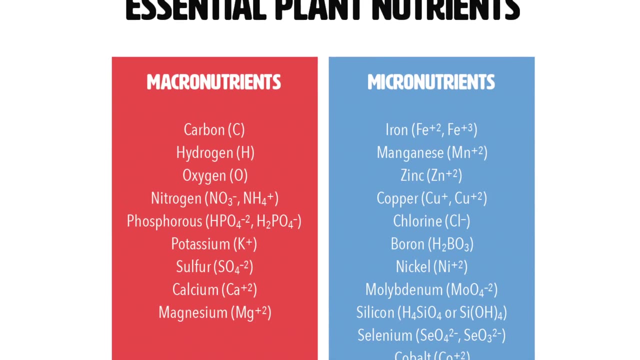 element to come in first and then, in this next stage of reactions, we need that element to come in, and that that's, that's totally true. but we need all of these elements, these nutrients available to, for proper plant health and function and even for proper photosynthesis. you know, for some of 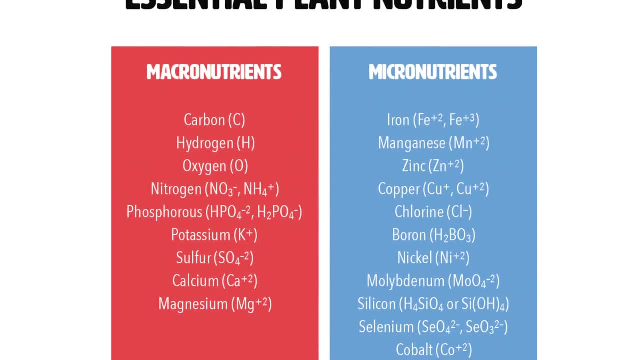 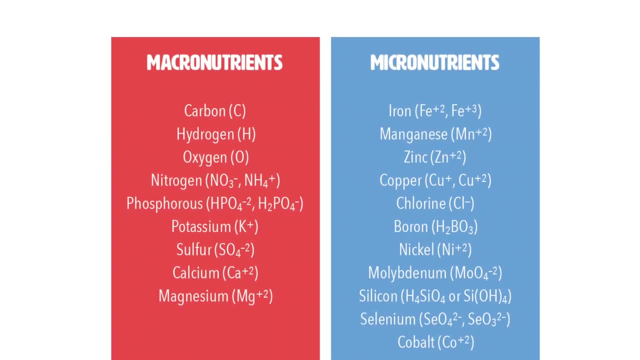 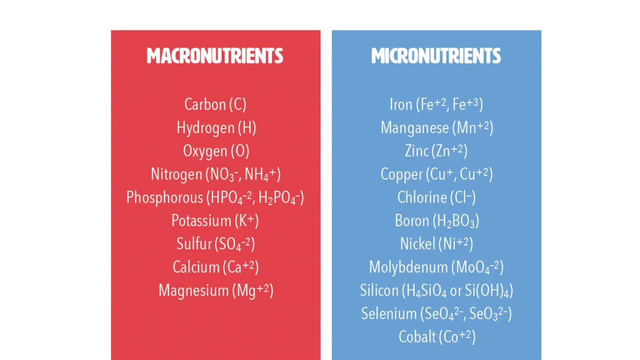 these, these nutrients, and it goes beyond that proper nitrogen fixation for some plants, but we need to have these nutrients there for those reactions to occur. so calcium is a macronutrient. it's incredibly vital. it's important for to boost plant immunity, but also growth and repair. so 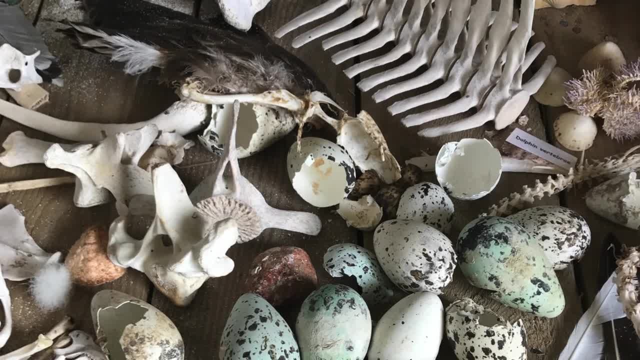 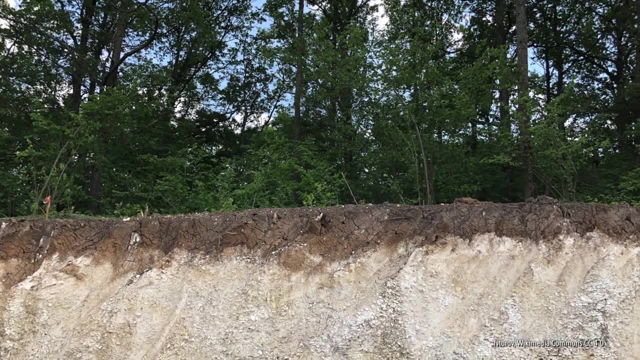 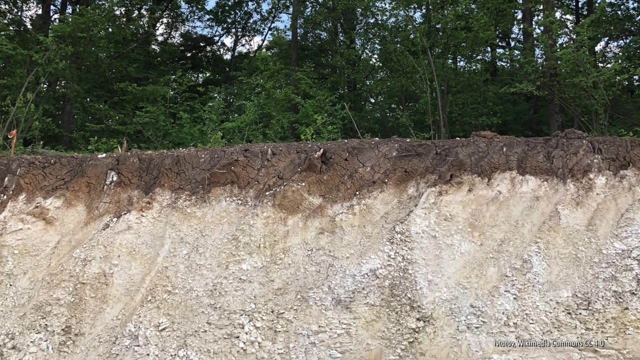 all the coral reefs, all the shells. they are made with calcium carbonate but, as i said before, limestone- right limestone- is predominantly calcite and arganite and also calcium carbonate. but it's that calcium carbonate that i want us to focus on for a moment, because we find that in the shells. 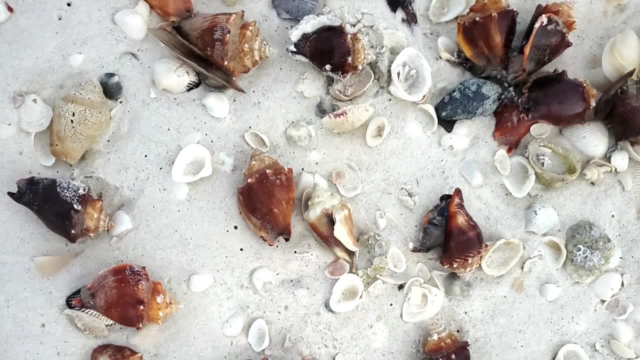 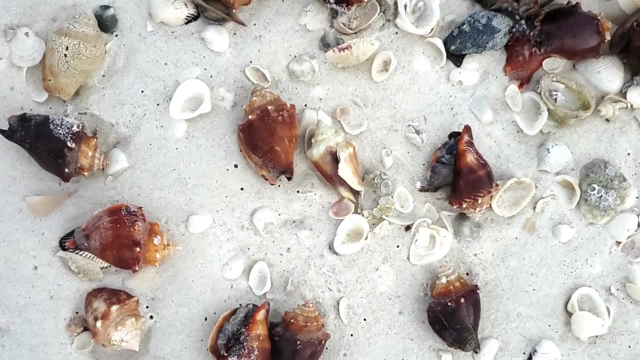 we find that in the tropical sands from the coral reefs, and this is why acidity in the oceans is such a big deal. because the acidity in the oceans is so important, because it's so important for the animal and its nurse philosophy- yeah, i agree. and and because all the the animals with shells. 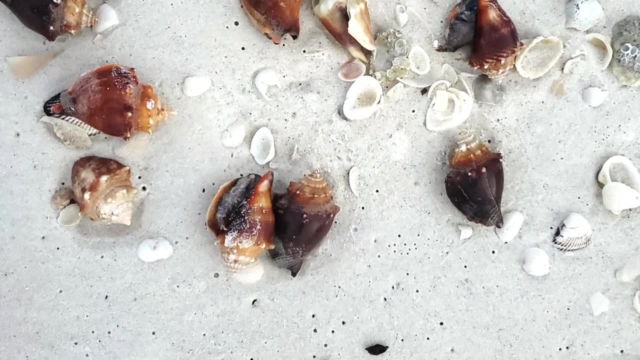 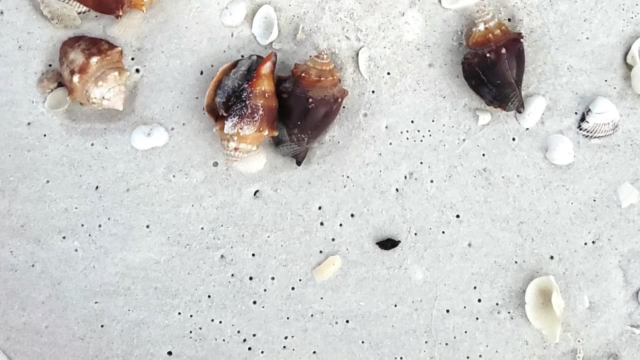 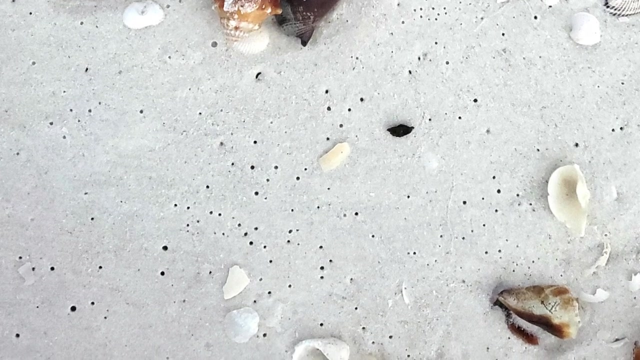 all you know, all of them are relying upon an alkaline environment to maintain the integrity of their shells and as soon as we raise the acidity, we we actually break those things down, we we start to acidify them and they start to solubilize. this is good to know for us in the 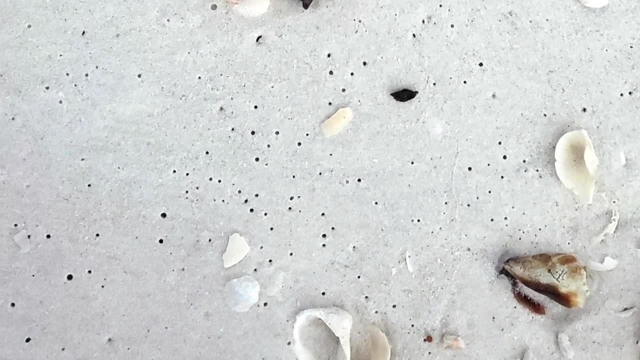 soil right that we need to make sure that we're in the right ph zone to unlock calcium in the soils for canadians. cause receiver இulfu chiar Cause. we need to make sure that we're in the right ph zone to unlock calcium in the soil for the달�ianians, in the channels for cyans, for canadians for نہ. 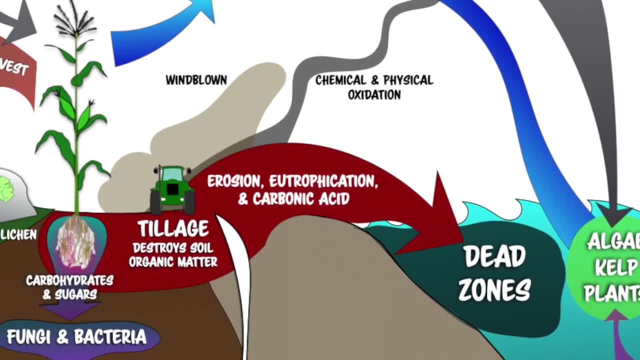 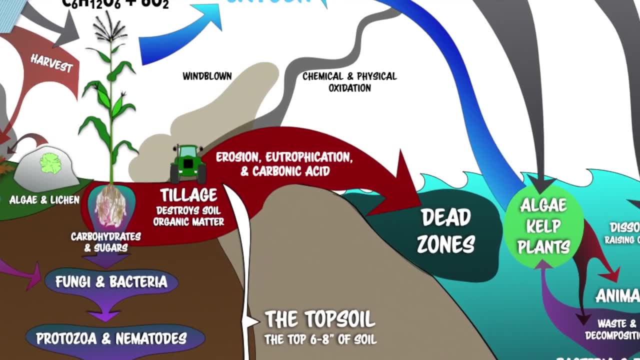 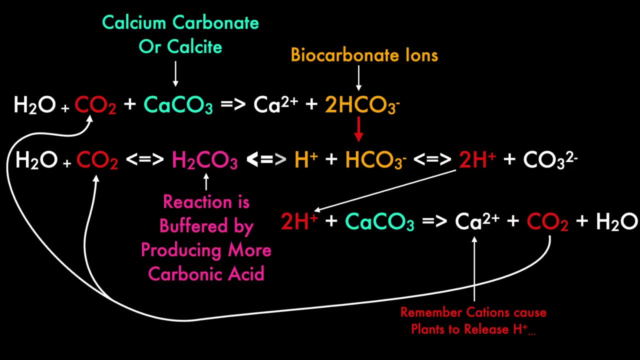 for us. But this also demonstrates why it's so incredibly important to keep the carbonic acid, the topsoil, runoff, because the topsoil running off is always combining with water and creating carbonic acids. The carbon is right, And so that carbonic acid, that's H2CO3 that combines with 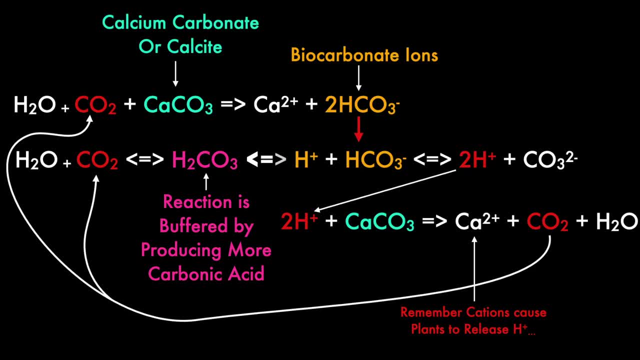 calcium carbonate, So CaCO3.. So as these things combine, we have a lot of CO2 being released, which again diffuses in the water and again becomes carbonic acid and continues the process of acidification. It's a runaway train effect, in fact, And it's the most dire environmental.